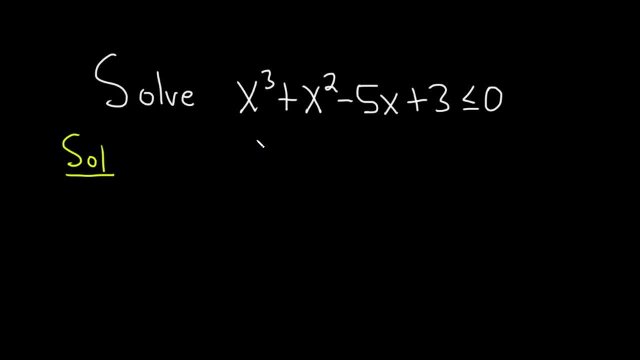 this. So what I'm thinking is I don't see a way to factor it by grouping. Usually, when you have four terms, you can try to like, factor something out so you get a common factor. but I'm not seeing that. So instead let's just see if we can find a 0 to this. So let's check to see if 1 is a. 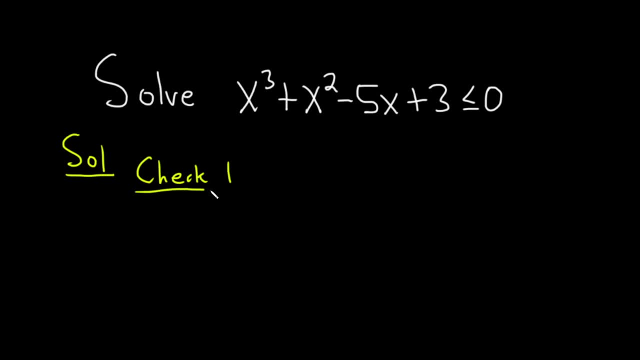 0.. So let's check 1.. And why 1?? 1 is always just a good one to check, because usually you know, on these problems 1 and negative 1 are good ones. So we have 1 cubed plus 1 squared minus 5. 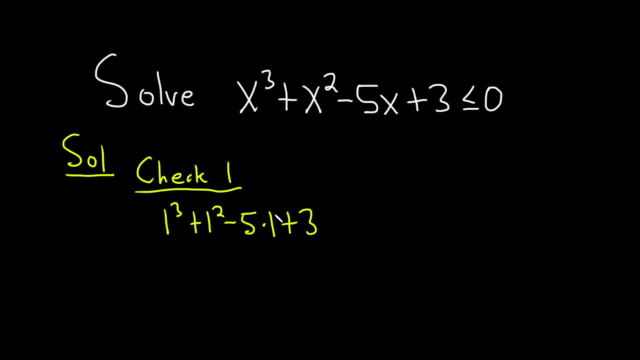 times 1.. 1 plus 3.. And basically we're just adding the coefficients. You can look at it that way too: If you add the coefficients and you get 0, then 1 is a 0. So this will be 2 minus 5 plus 3.. So this: 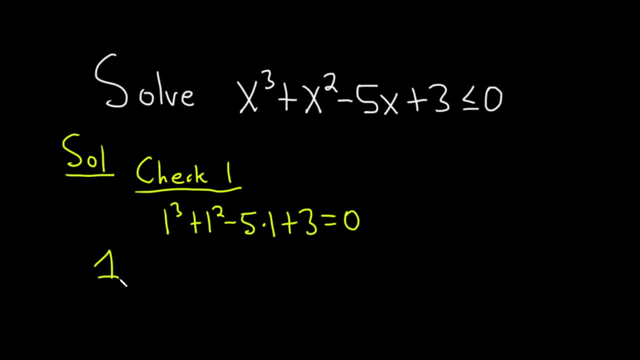 is 0.. So 1 is a 0.. 1 is a 0. And so therefore we know that x minus 1 is a factor is a factor, And so if we divide by x minus 1,, therefore, the remainder will be 0.. So let's do that. 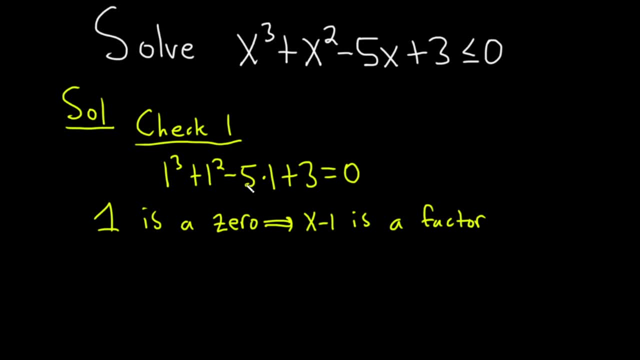 And the next step: we're going to divide by x minus 1.. And to do that we basically flip the sign, put a little bracket here and we move to synthetic division. We write down the coefficients 1, 1, negative, 5, and 3.. And then we draw a line. Let me go through all of that again from the 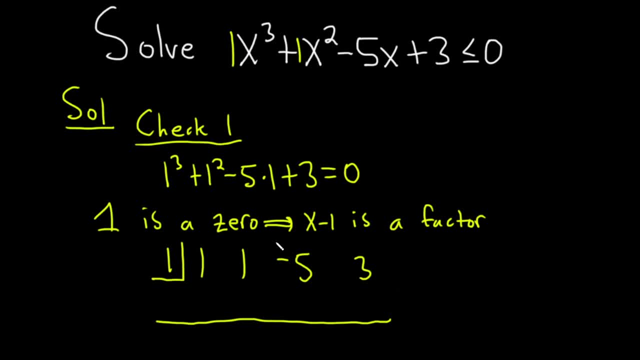 beginning, Because there's a lot of information here And if you're not familiar with some of it, it might seem like a lot. So we're trying to solve this inequality, So we're trying to factor it somehow. Factor by grouping is usually a good idea when you have four terms. However, in this case, 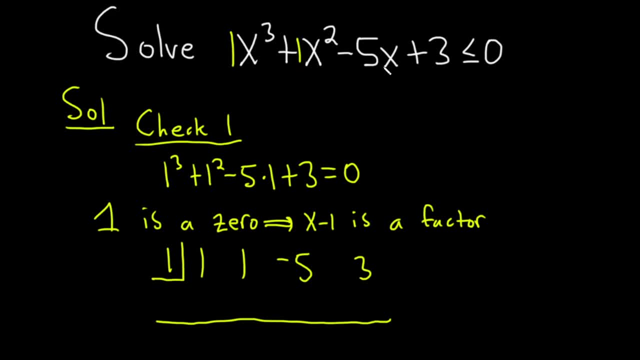 I don't see something nice that we can pull out. that's going to leave us with a common factor. So we can try to use the rational roots theorem, But instead, even before going to that, we can just check one right away directly. 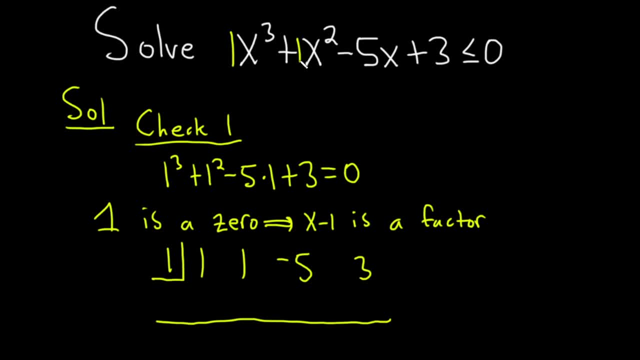 To check one, you can just add the coefficients. 1 plus 1 is 2.. Minus 5 is negative, 3. Plus 3 is 0. So 1 is a 0. Here I showed it by evaluating the function, by plugging in 1 and showing it's. 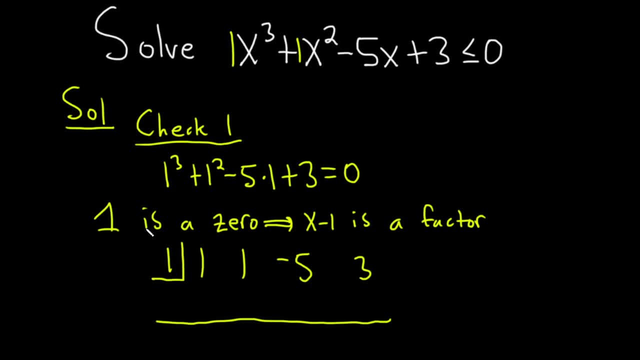 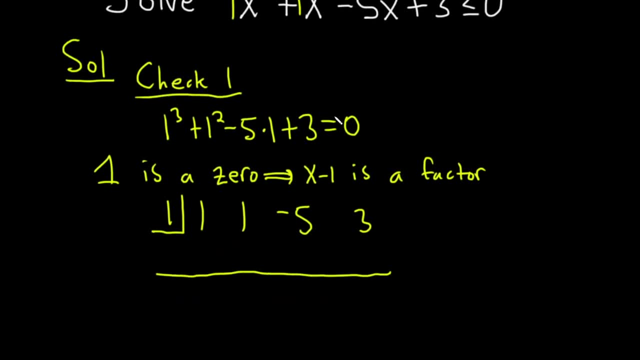 equal to the same thing as adding the coefficients Whenever 1 is a 0, x minus 1 is a factor, And that means if you divide by x minus 1, the remainder is 0. And you can use that to factor the rest of. 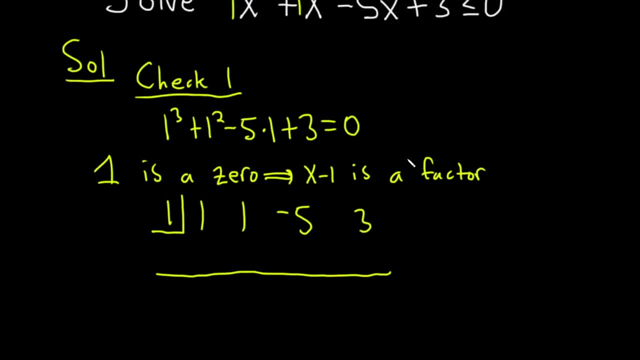 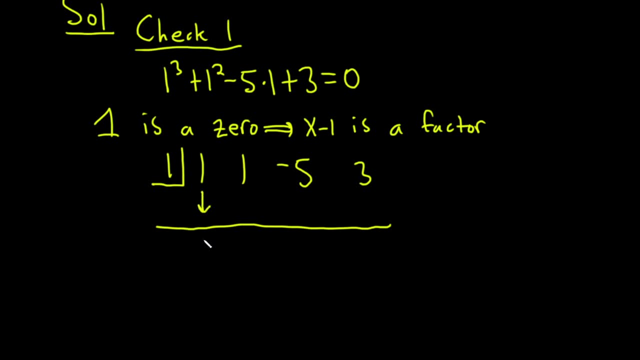 this polynomial. So we wrote down the coefficients. Let me just double check them: 1, 1, negative 5, and 3.. The first step in synthetic division is to take this number and bring it down So 1.. And then we multiply 1 times 1 is 1.. We add 1 plus 1 is 2.. Multiply 2 times 1 is 2.. 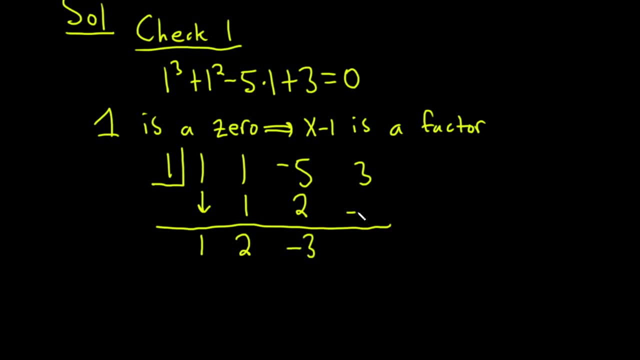 We add, We get negative 3.. Multiply, We get negative 3.. We add And we get 0, which means that 1 is a 0, which we already knew. However, now we know that our original polynomial is really x. 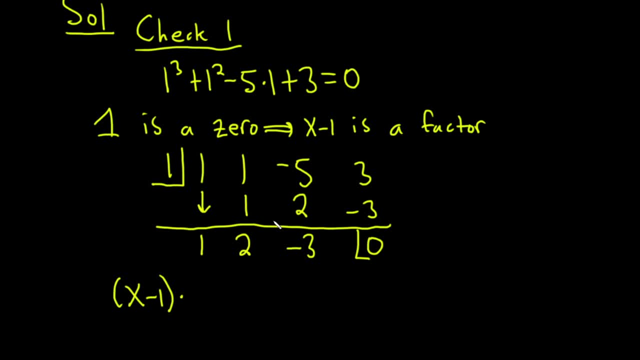 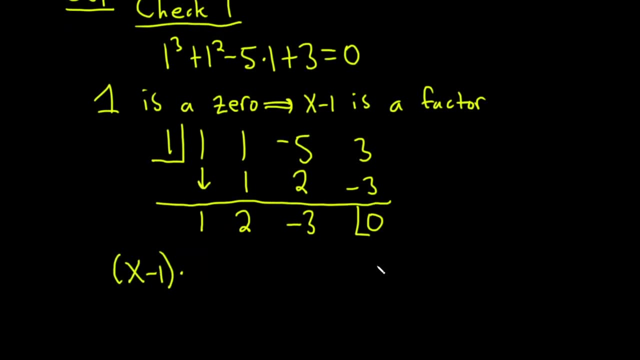 times. And then here it's going to be 1 less in degrees, So this is a 3.. So this is going to be a quadratic. So it'll be 1 times x squared, which is x squared plus 2 times x minus 3.. So it's 1. 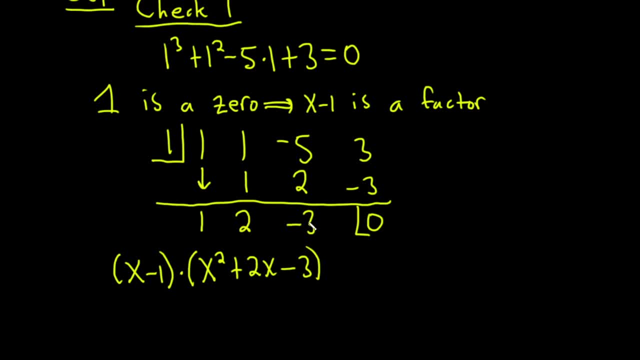 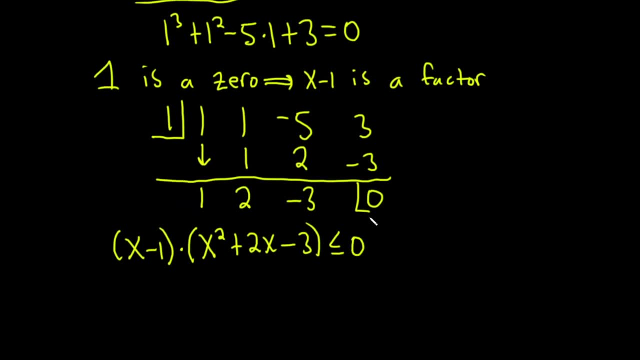 times x squared, 2 times x minus 3.. And we want to see when this is less than or equal to 0.. That was the original question, right. Less than or equal to zero? Okay, let's try to factor it some. 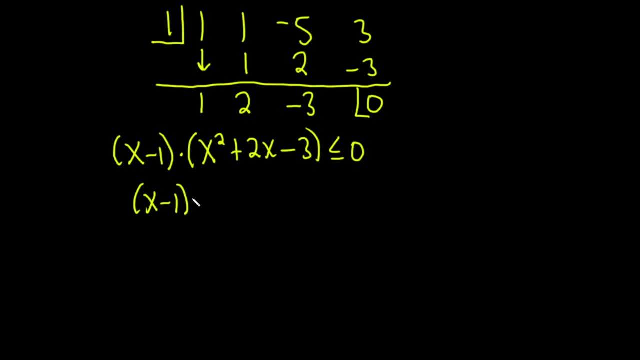 more. I don't know if it will. I have not done this problem. So let's see here. I think this factors. let's try it. I'm just going to try to guess. So two numbers that multiply to three, well, one and three, or rather negative three. So let's make the three positive. 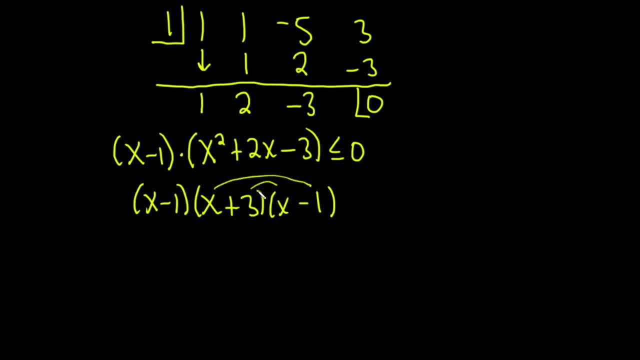 and then 3x plus a negative x. the inner and the outer, give you the middle term, always 3x plus negative x is 2x, And we want this to be less than or equal to zero. Look at this: 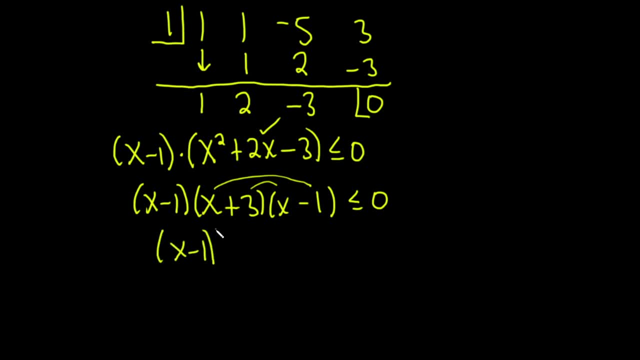 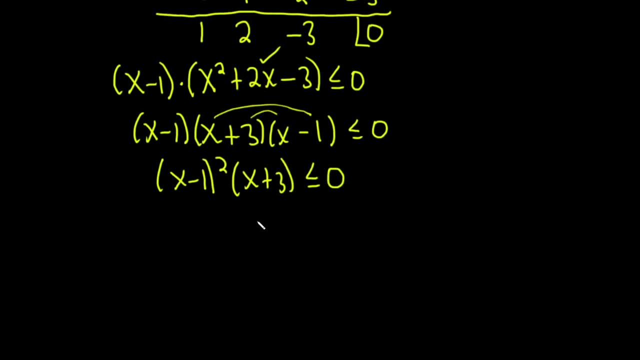 we have x minus one. twice. this is really x minus one squared, x plus three less than or equal to zero. So x minus one squared is never going to be negative. okay, It's never going to be negative because it's being multiplied by x minus one. So we want this to be less than or equal to zero.